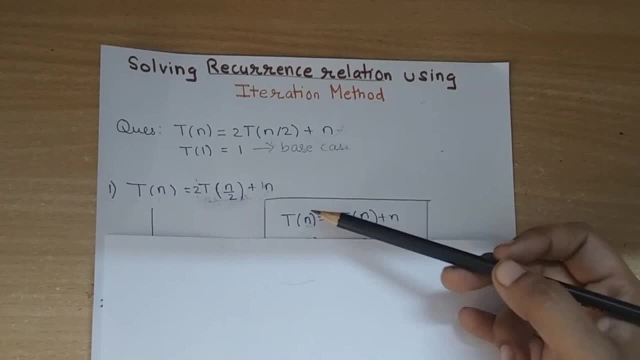 out the value of tn. we have to find out the value of tn. So we have to find out the value of tn. Now, in phi n by 2. what you have to do is, in place of n, put n by 2.. Just replace n with. 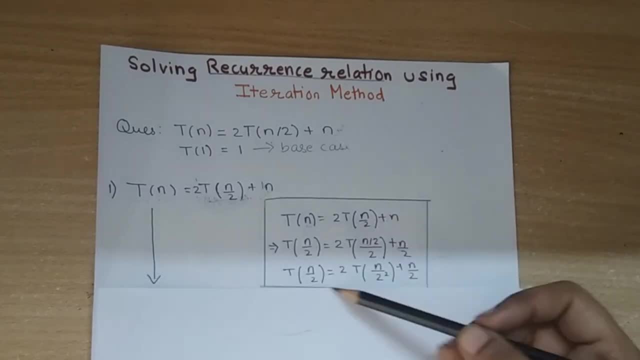 n by 2, and the value that you will be getting is this: tn by 2 is equal to 2, into tn by 2 square plus n by 2.. Now, as you have got the value of tn by 2, replace it or substitute. 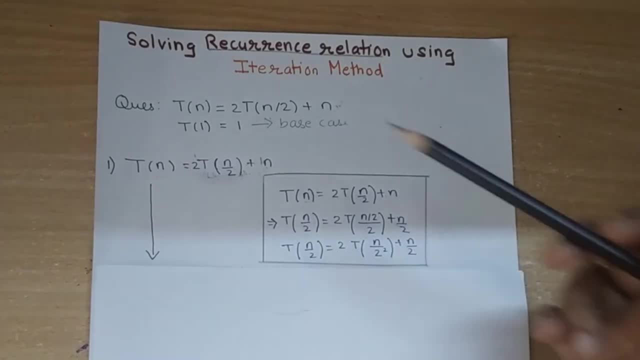 it back in the main equation of tn, So the value of tn will now become this: After replacing the value of tn by 2, you can replace it with this: After replacing the value of the original Principality of tn, the valuation of tn is will now become this: Tn is a equal to 1, saying: 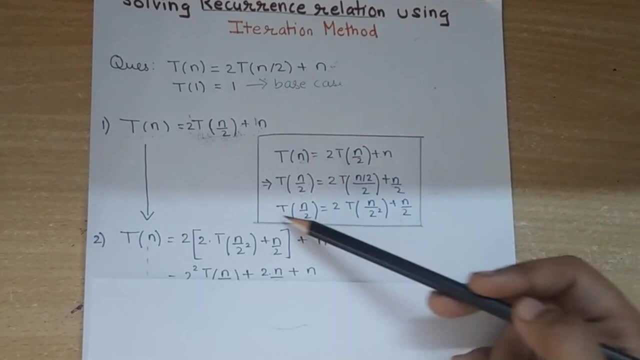 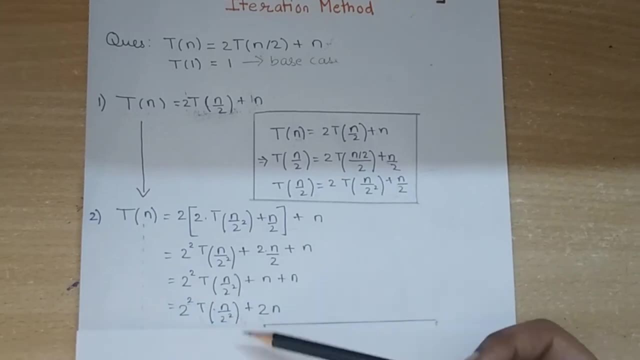 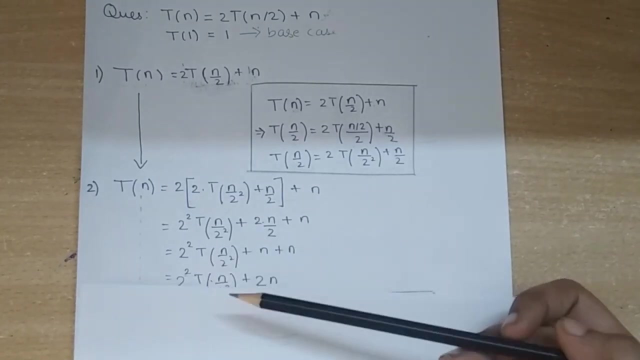 n by 2 with its expanded form. now open the brackets, cancel out the common terms, and this is the value that i have that i will be getting. so notice that i have not written 2x2 equal to 4, which is obvious, but i am doing it in this way to search for patterns. notice when: 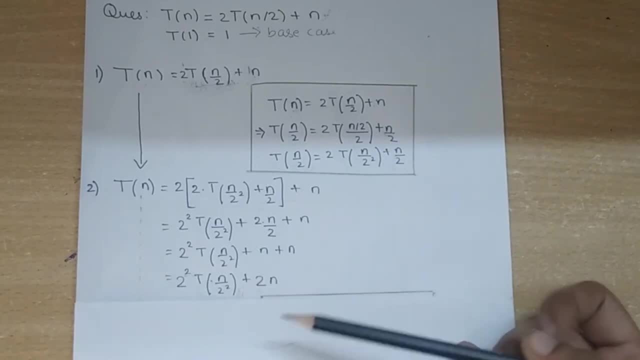 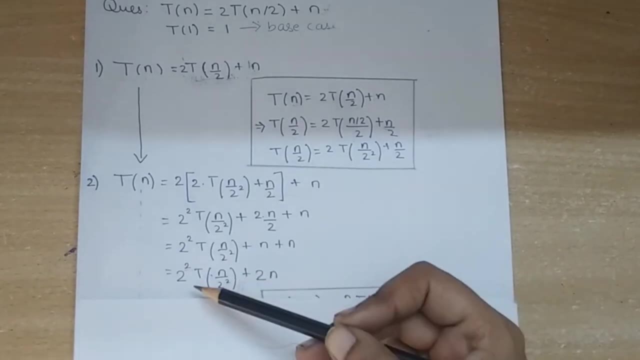 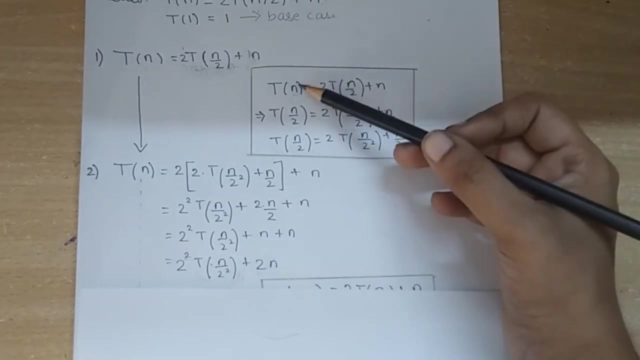 you solve questions of iteration method, you have to look for patterns. only then you can simplify your final equation. so now again repeat the procedure that i did before: find out the value of this sub problem. to find this value, simply put n by 2 square in place. 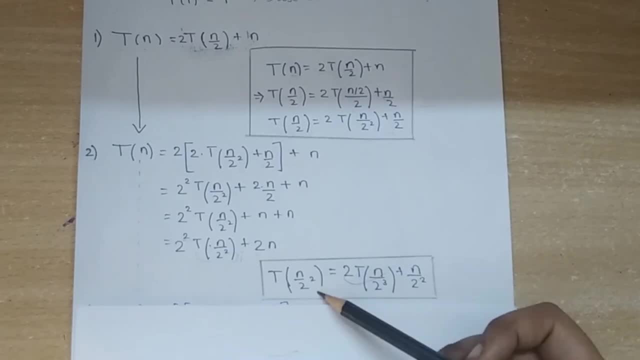 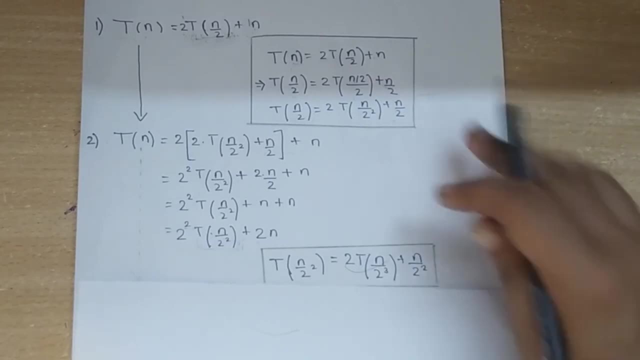 of n here and you will get the value of tn by 2 square. so i have just replaced the value of n with tn by 2 square and this is the value that i have got. so now place this value back in the main equation. substitute it back. 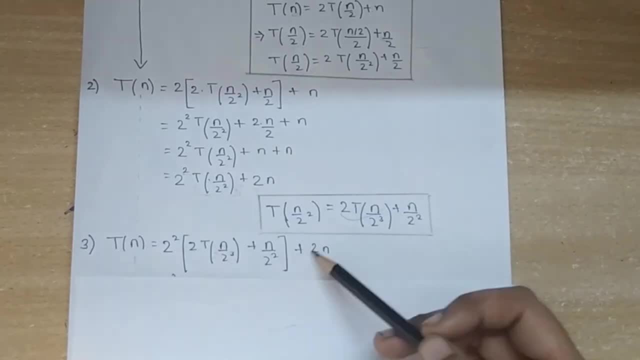 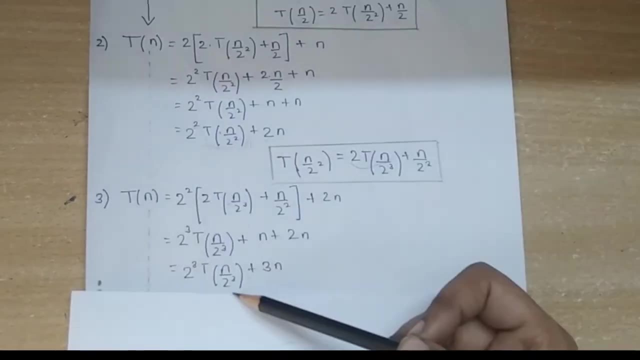 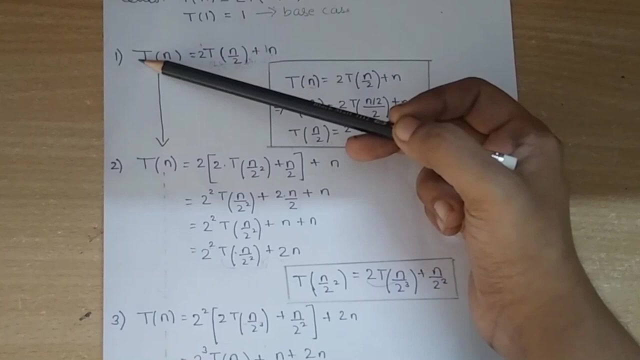 and this is the final equation that will come now: open the brackets, simplify it, cancel out the common terms, and this is what i get. so, as you can see, i have found out a pattern. i started with my first step and the coefficient of 2 was 1. sorry, the power of 2 was 1 and 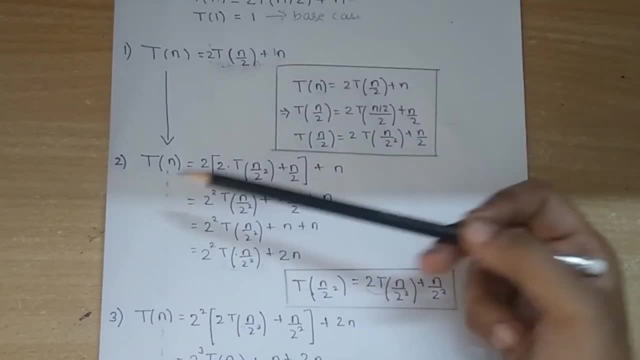 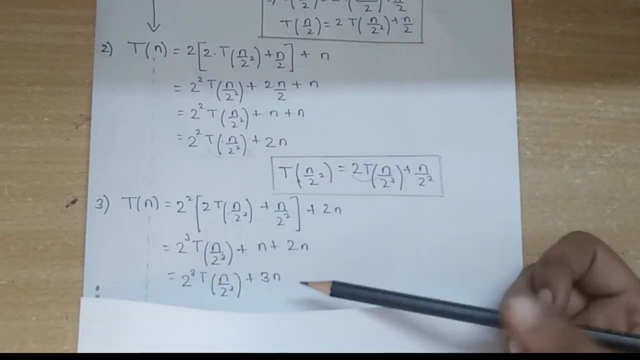 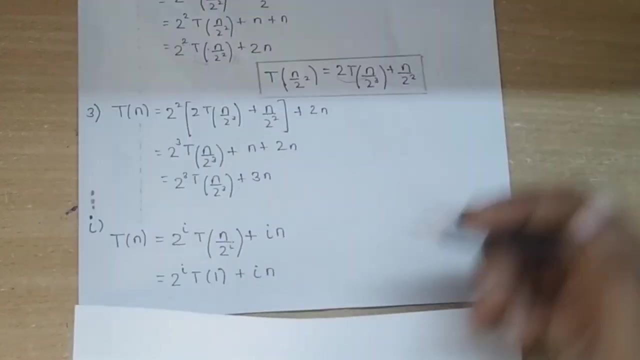 the coefficient of n was 1. then i did it my second time. the power of 2 was 2, the coefficient of n was 2. when i did it third time, the power of 2 was 3, the coefficient of n was 3. so what if i do it? i times, i know. 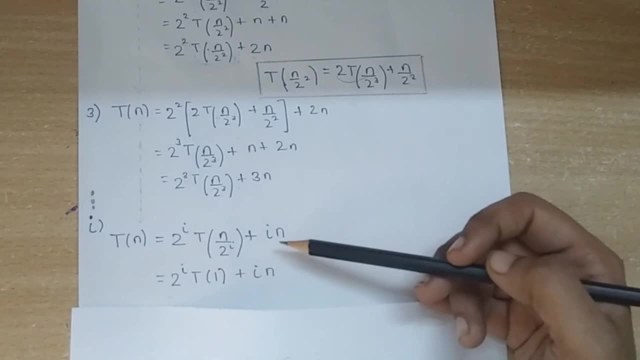 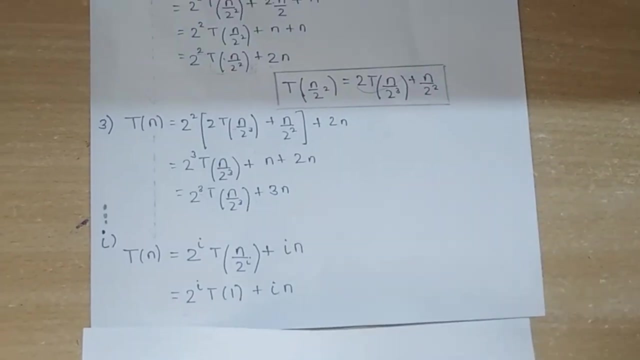 with the pattern that the power of 2 will become i and the coefficient of n will become i. but the question is: how long do i have to keep on doing this? i have to keep on doing this till my sub problem reduces to 1. as you can see it, as i am expanding the terms, my 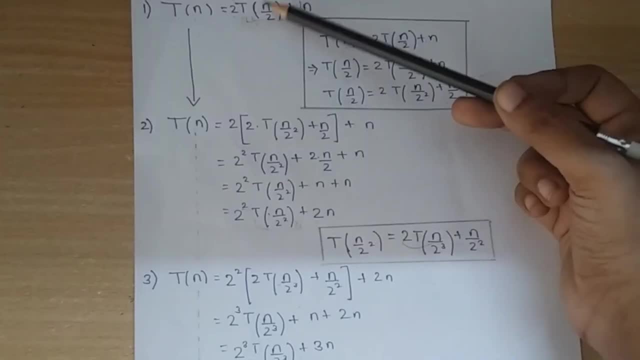 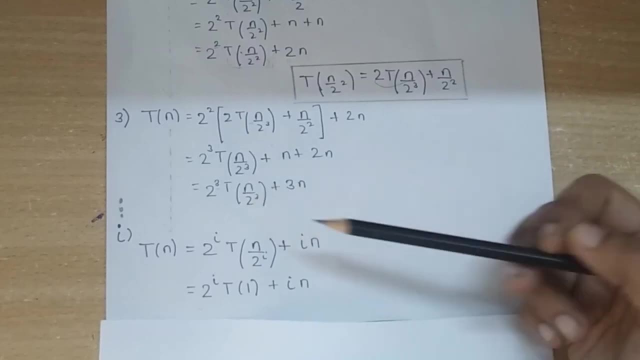 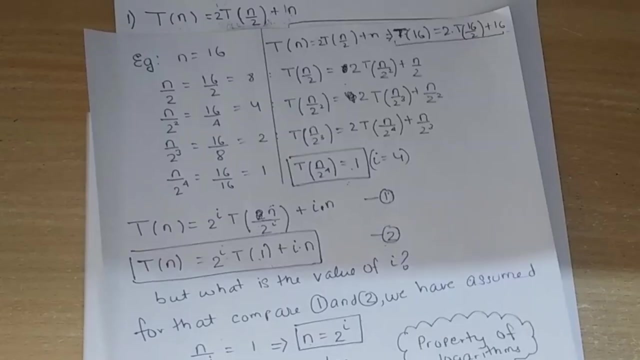 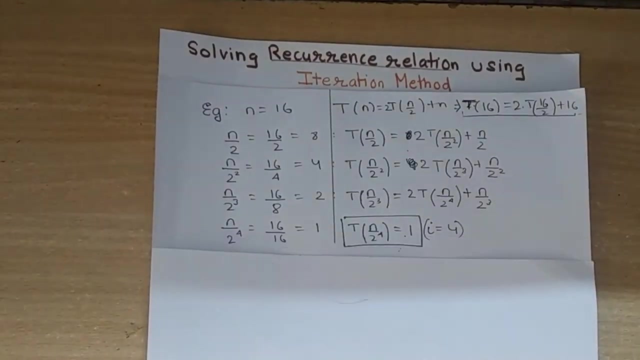 sub problem is: reducing n by 2 is a bigger value, then n by 2 square is a reduced term. then i reduce it further: n by 2 square cube. so let's understand it with an example. let's suppose that i knew the value of n, which is 16. i know that when i divide it by 2, it 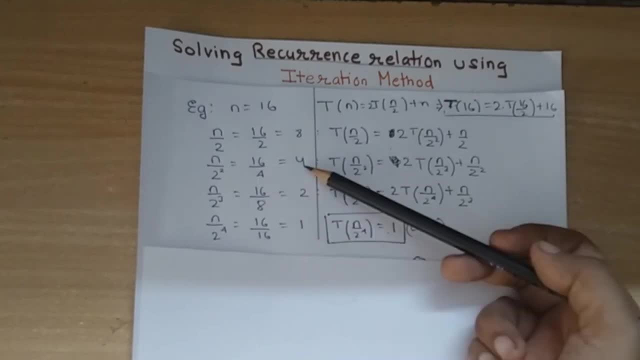 becomes 8. when i divide it by 2 square 2, it becomes 4. when i divide it by n square 2 square 3, it becomes 2. n divided by 2 square 4 becomes 1. so my sub problem is reducing. and finally, 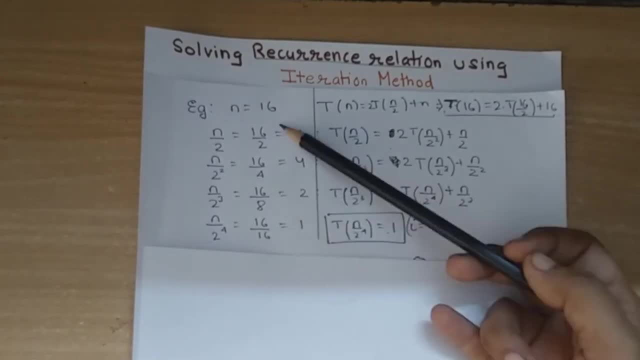 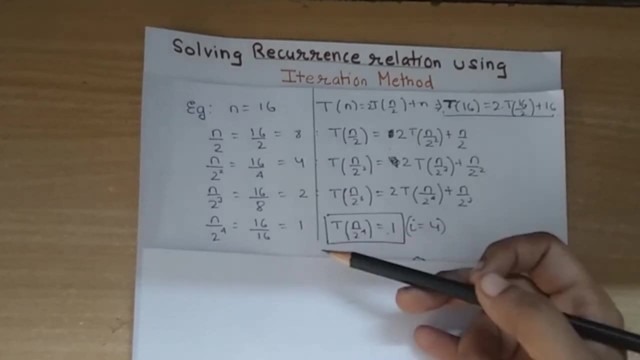 it will reach 1. so i know that when n is 16 i have to take i is equal to 4 that i have. that means that i have to do it 4 times, expand it 4 times and my sub problem will reduce to 1, which is when i will terminate, which is when i will stop expanding it further. but 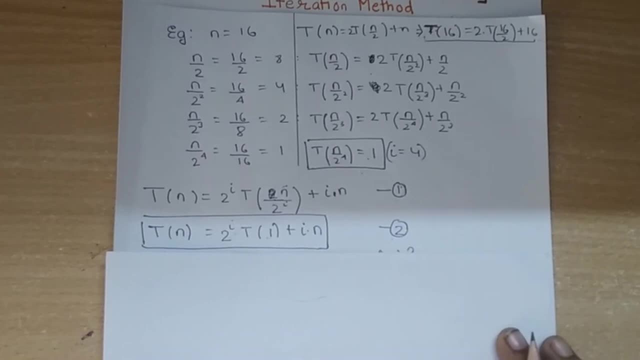 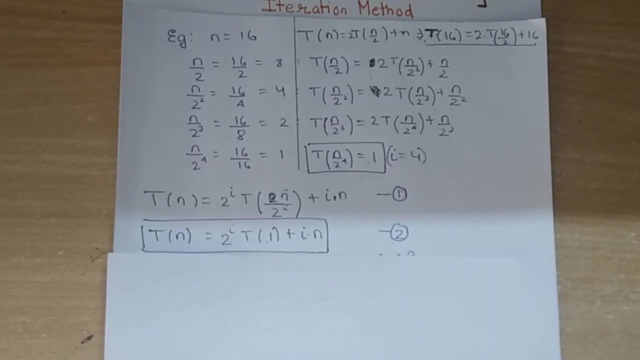 i don't know the value of n in general. right, i have to take out a variable. i'm assuming that when i don't know the value of n, i have to keep on expanding it. I times when my sub problem, n divided by 2, raised to, i will reduce to 1. this is my assumption. 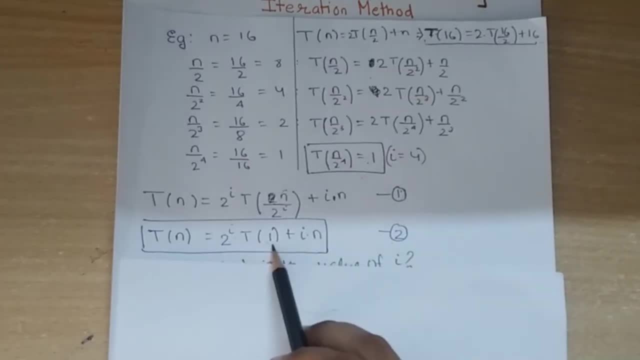 So this is where i will get 1 when i do it i times. and when i do it i times, the power of 2 will be i and the coefficient of n will be i. but the problem is that there are two variables here: n and i. i don't know the value of i, but in iteration method the final equation should: